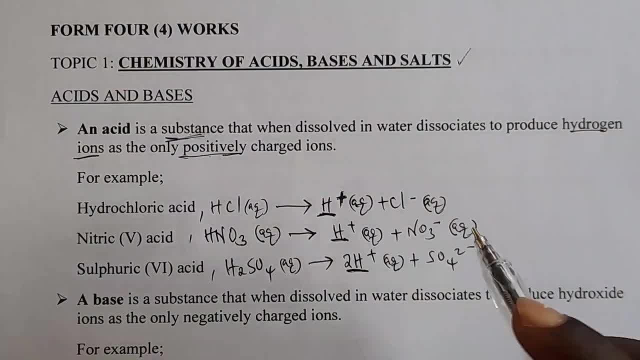 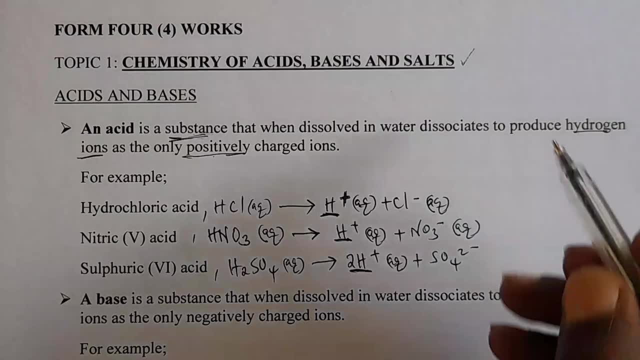 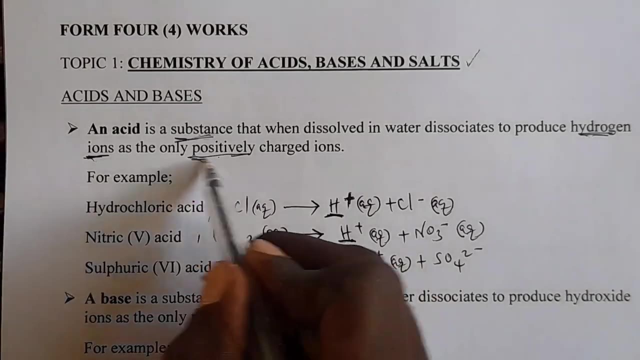 H3O18, H3O19, H3O20, H3O23, H3O24, H3O24, H3O25, H3O27, H3O27, H3O24, H3O27, H3O27 ions. then you replace with hydroxyl ions, the definition will be okay. then you check positively. 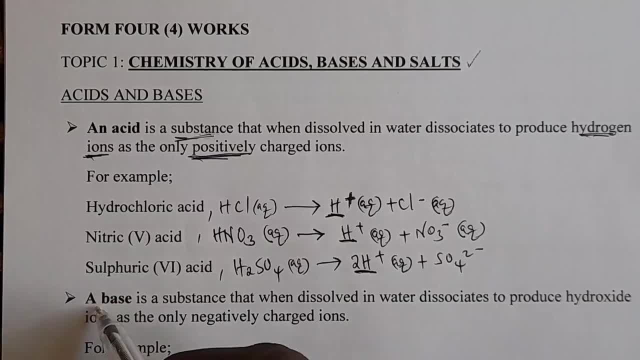 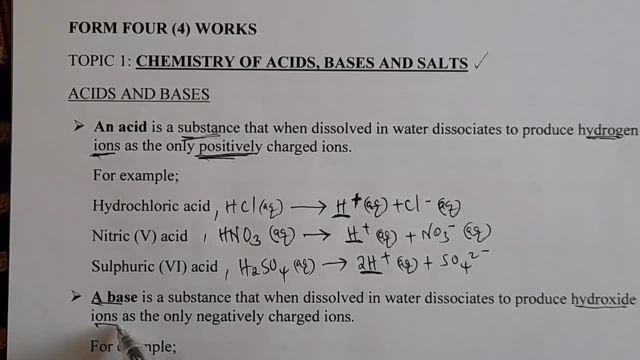 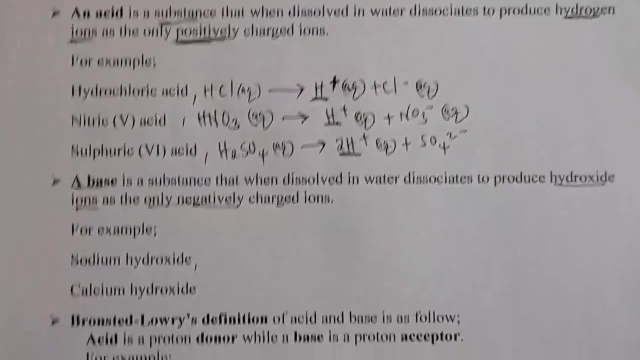 charged ion, then you replace with negatively charged ions. so what's a base? a base is a substance that, when dissolved in water, dissociates to produce hydroxide ions as the only negatively charged ions. for example, sodium hydroxide. how do you write sodium hydroxide, sodium hydroxide? 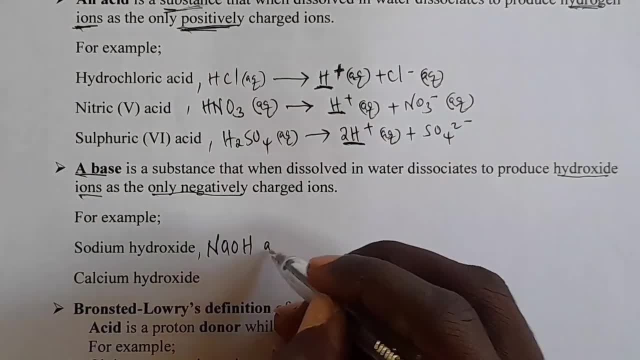 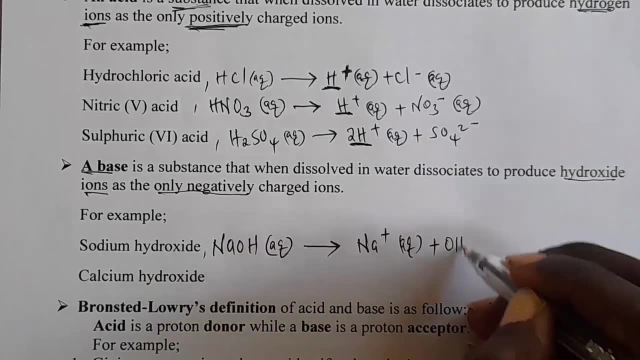 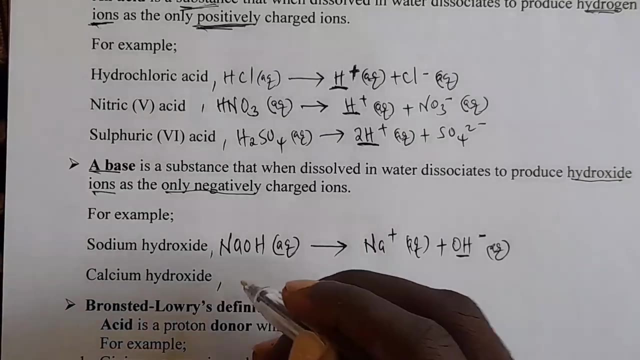 we are going to write naoh. when it dissolves in water, it dissociates, producing sodium ions and also hydroxyl ions. so we are having hydroxyl ions as the only negatively charged ions. so sodium hydroxide is a base. let's go for calcium hydroxide. it's written in chemical formula. 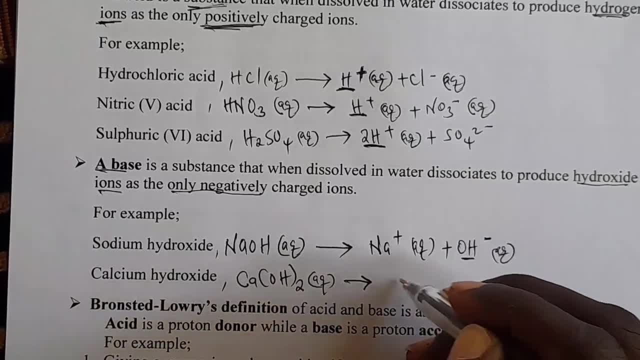 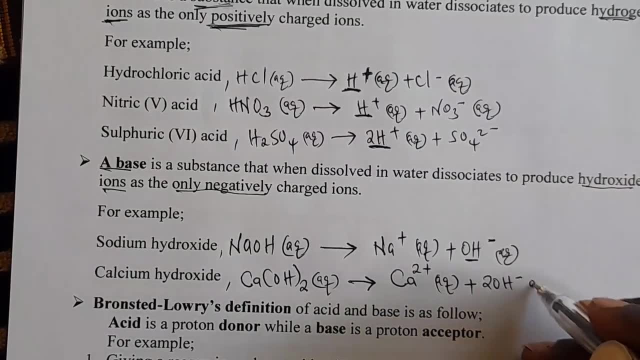 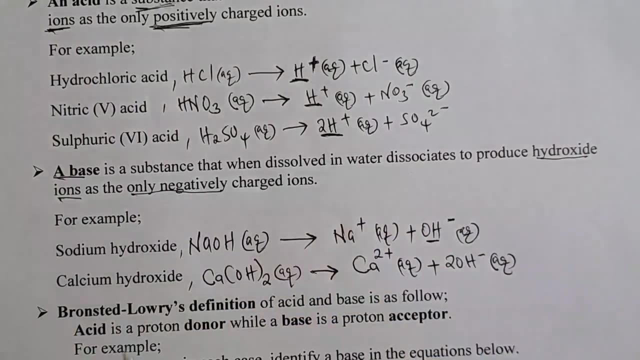 like this. calcium hydroxide dissociates in water, producing calcium ions occurs, and also two of hydroxyl ions which are ruckus. so we are saying a base is a substance, when dissolved in water dissociates to produce hydroxyl ions as the only negatively judged ions, as you can see in our two examples. 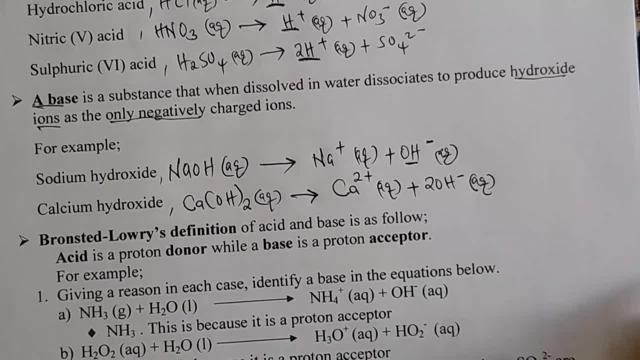 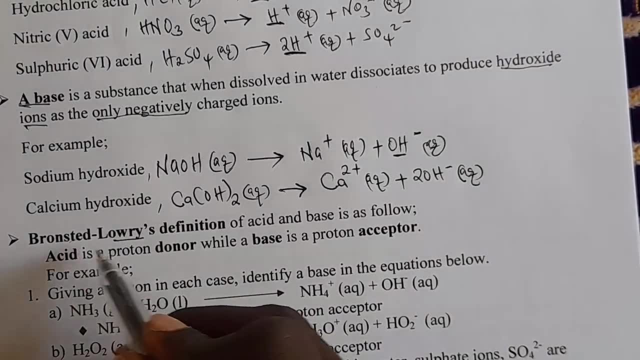 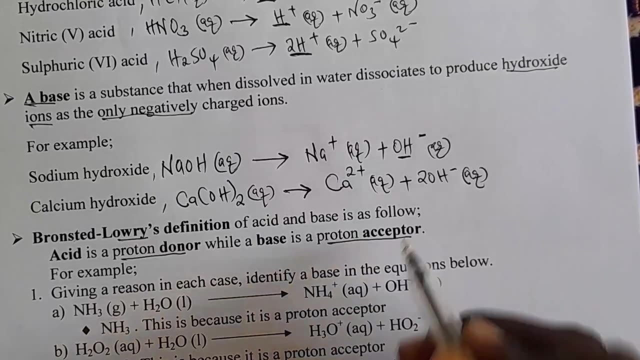 here so we can be told again or ask to define acid and basis using Brosted-Lowry's definition. so, according to Brosted-Lowry's definition, acid is defined as a proton donor, while a base is defined as a proton acceptor, for example. let's go to the first one. we are told. 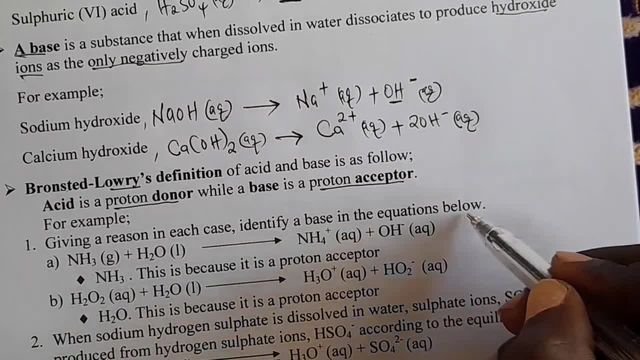 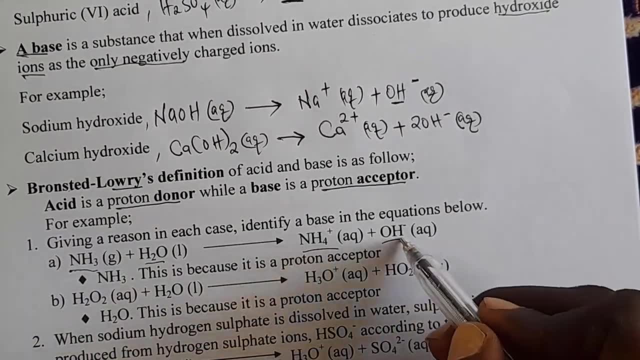 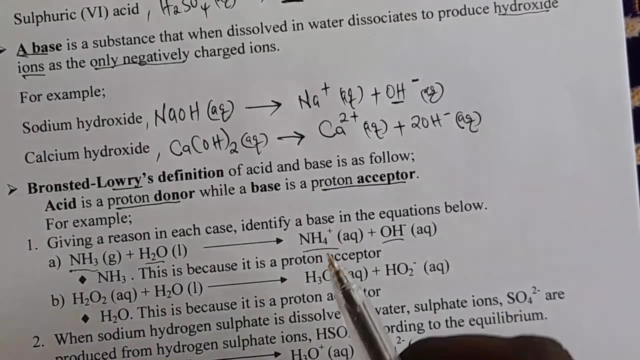 given a reason, in which case identify a base in the equation below, in the questions below. so we are having here ammonia gas, ballast water, giving you ammonium ion and also hydroxyl ion. so if you are told, identify a base or an acid in such a question, you are supposed to pick your. 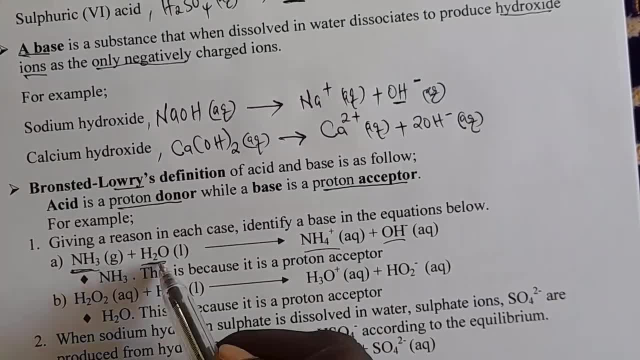 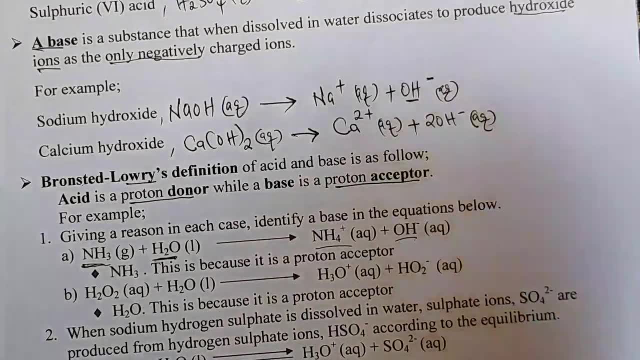 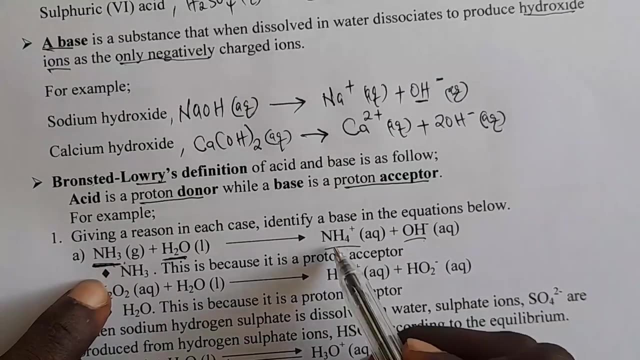 answer or your response, from the reactant side. the reactant side only. if you put, if you pick from the product side, you will be totally wrong. so let us see now, start with ammonia. ammonia is NH3. check now NH3, the number of protons of hydrogen with the product side. so here i'm. 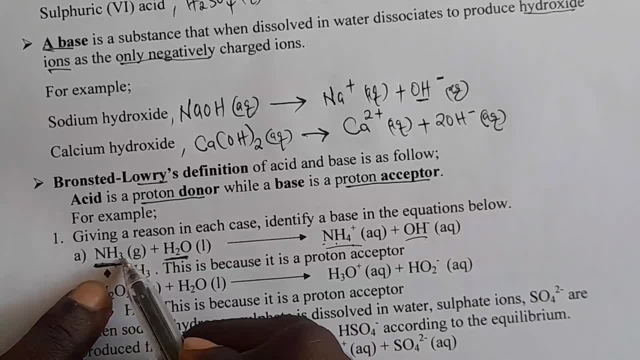 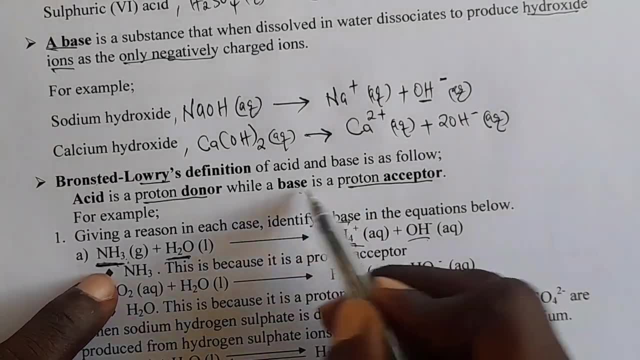 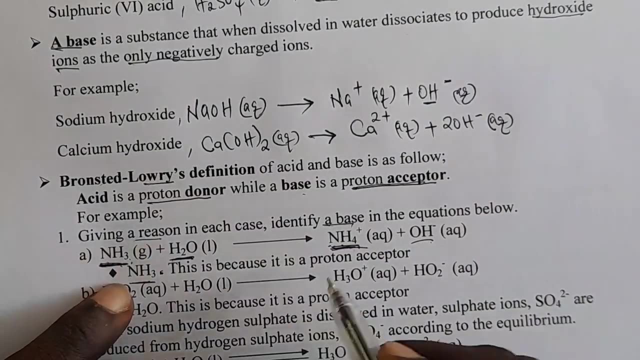 having NH4. that means it was NH3. it has. now it has accepted a proton. so what have we said about a base? we said a base it's a proton acceptor. so that means ammonia is the base reason. because we are given a reason it is a proton acceptor. or you can say: this is because ammonia gas accepts a. 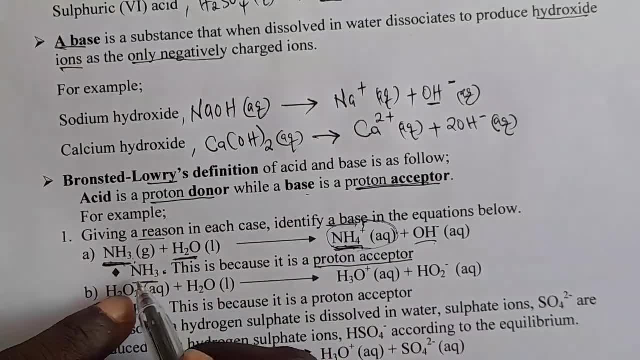 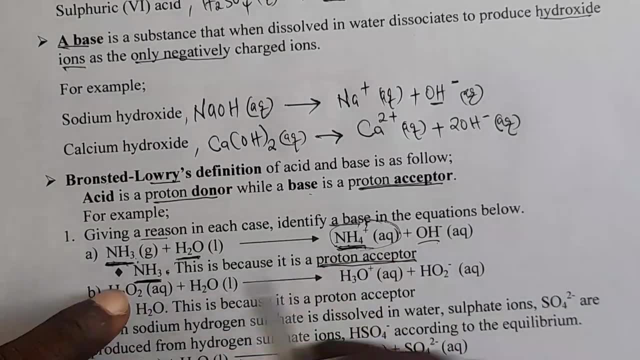 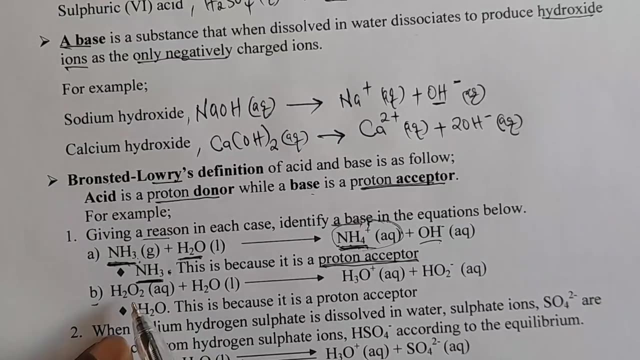 proton from water to form ammonium ion. so the answer will be ammonia gas. reason this is because it is a proton acceptor. or you can say this is because ammonia gas accepts a proton from water to form ammonium ion. let's go to the example number two here, this equation. we are told the same. 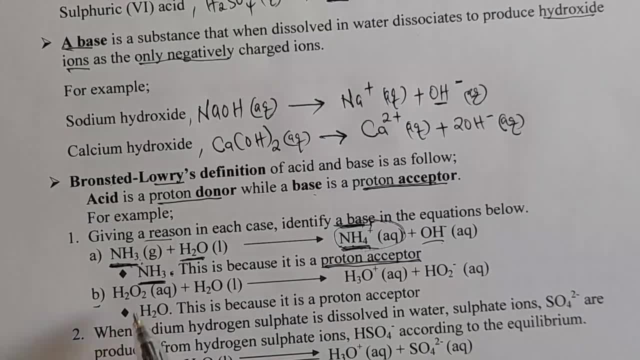 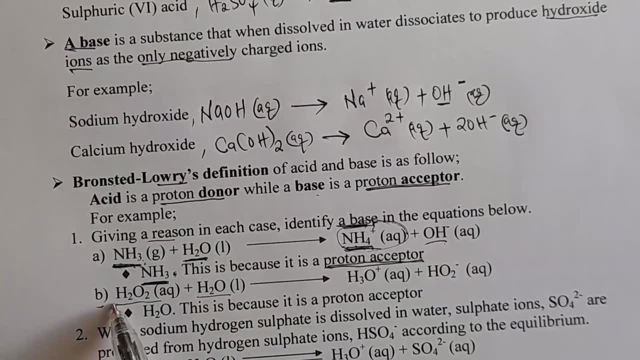 identify the base while giving a reason: hydrogen peroxide and also water. which one is a base? so we are going to see hydrogen peroxide, it is H2O2, but when you check here it is H. there's no two there. that means it was minus one. 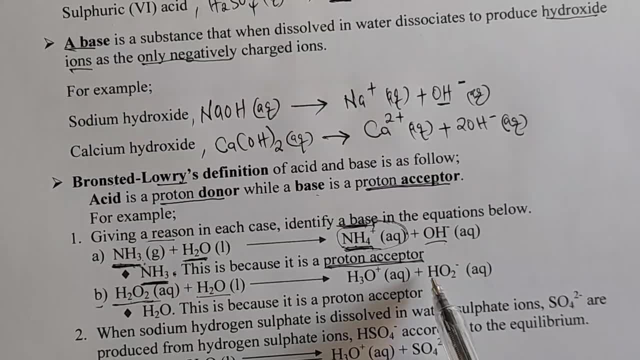 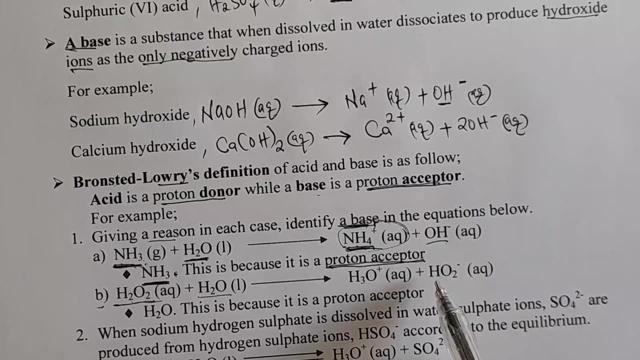 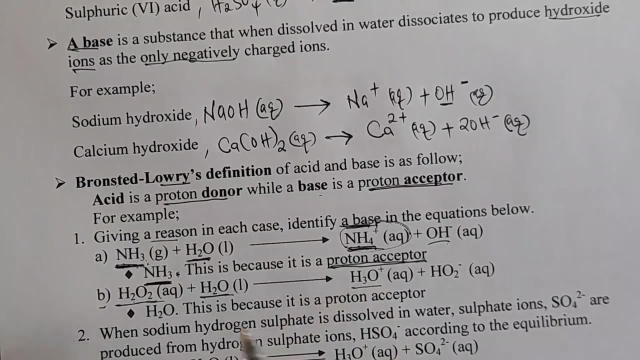 so it has now given out. so it's not a base, because a base accepts or receives a proton or hydrogen, but not gives out. so check water here H2O, but here i'm having H3O, that means H2O, that means H3O and H2 is a base because it has accepted a proton from the hydrogen peroxide. 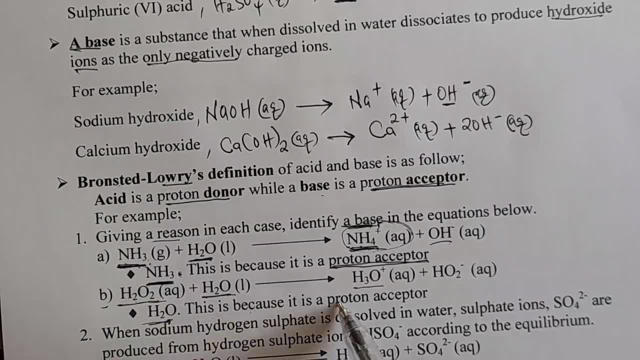 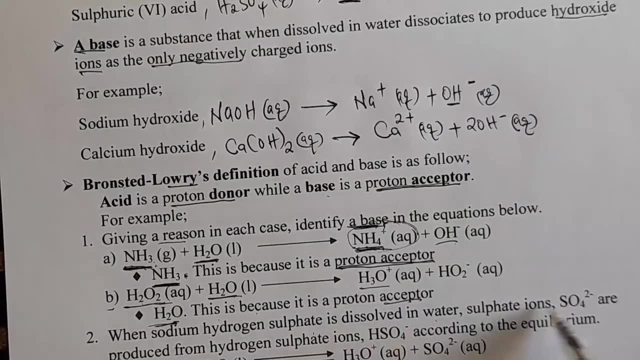 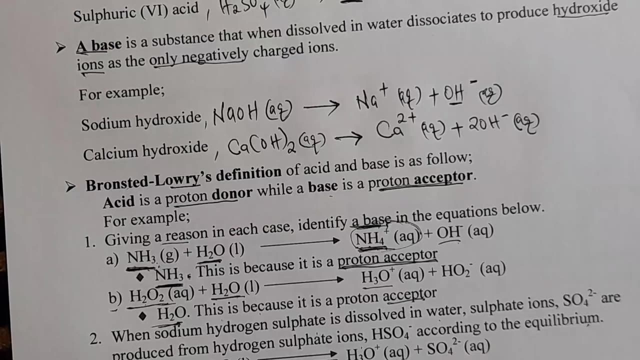 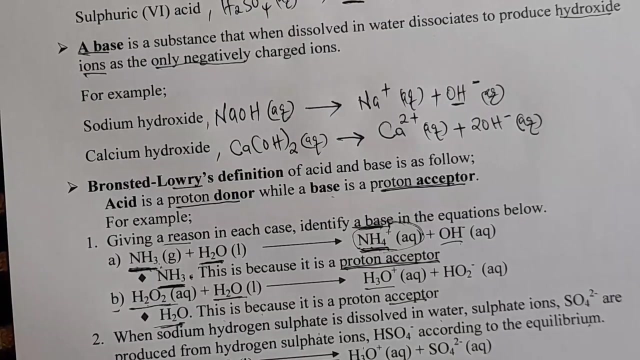 so water is our base reason. this is because it is a proton acceptor. okay, let's go. example two: when sodium hydrogen sulfate is dissolved in water, sulfate ions are produced from hydrogen sulfate ions according to the equilibrium. so this equation, you are seeing hydrogen sulfate ion plus water. it is in equilibrium, reversible reaction. we are having here hydronium ion and also 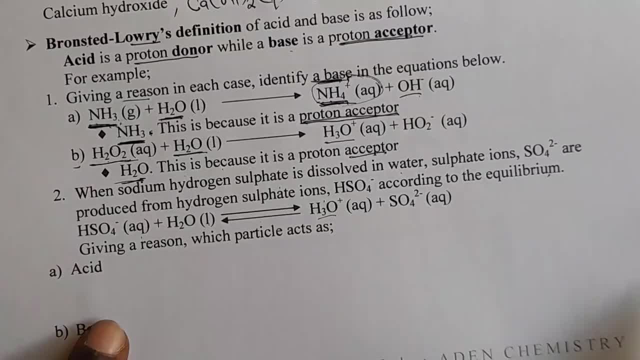 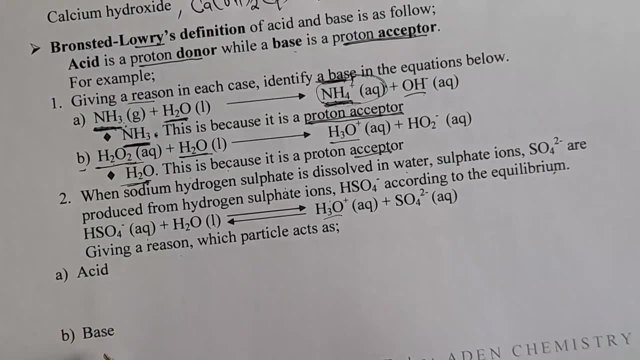 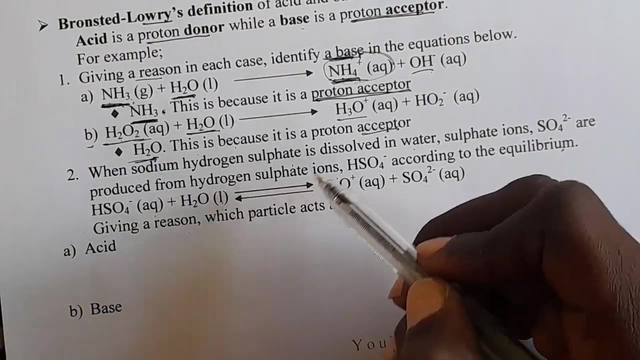 sulfate ions. okay, sorry, that's the question. so we are told, giving a reason, which particle acts as an acid and a base. so if you come across such a question, and it's irreversible- you expect the teacher to tell you which side you are going. is it backward reaction or forward reaction? 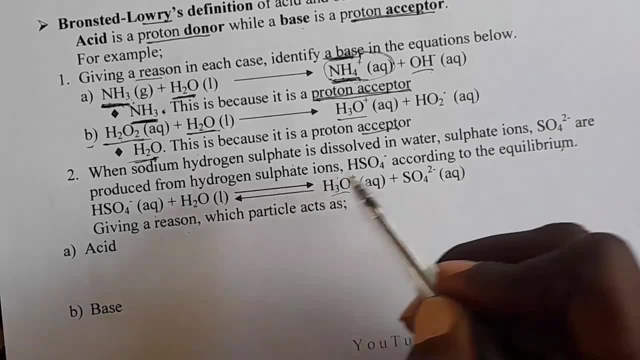 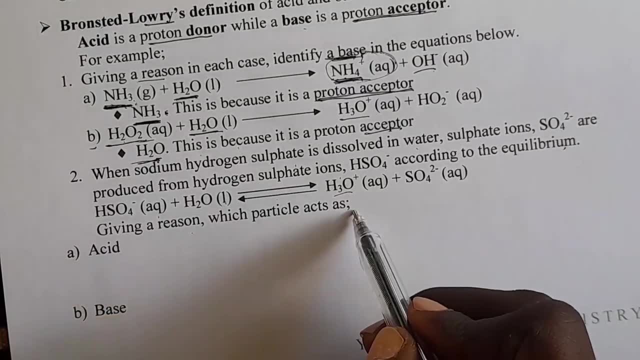 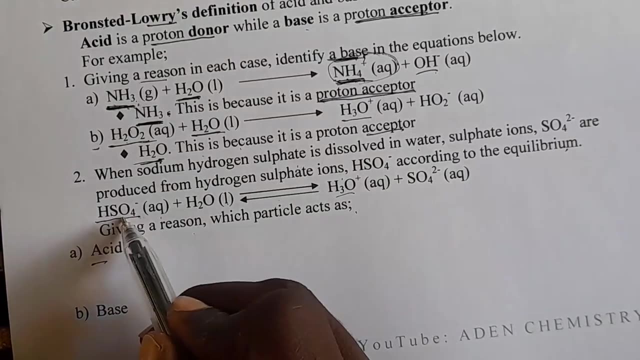 if he doesn't disclose or tells you to decide, you are supposed to take your answer as if he has asked you on the forward reaction. so, given a reaction, which particle acts as an acid? let's check here now: hydrogen sulfate ion. so hydrogen sulfate ion, let's check on the borax side we are having 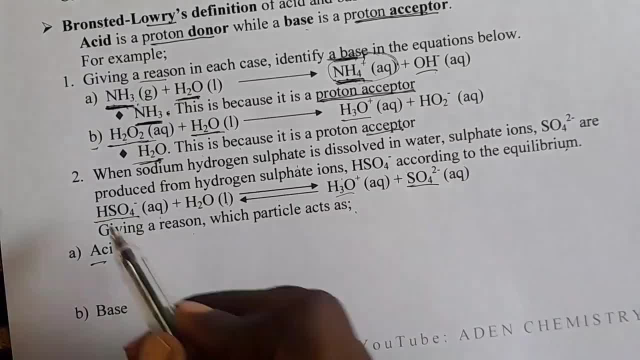 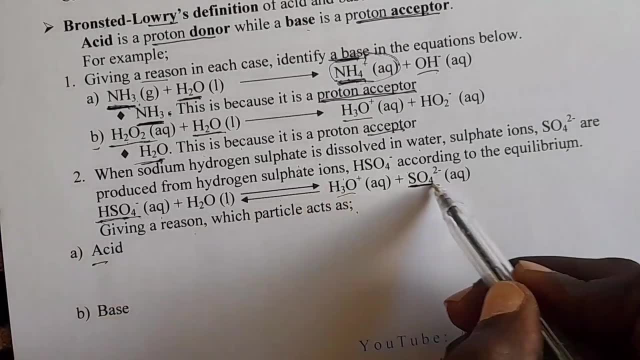 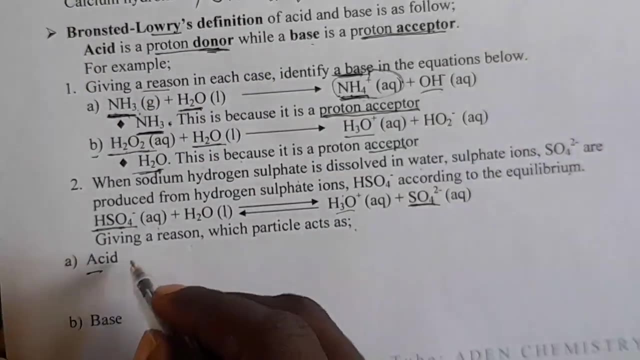 so4 here. that means we are missing the hydrogen there. so that means hydrogen sulfate ion donates the proton, that hydrogen proton, and becomes sulfate iron. so what have we said about acid? we said acid is a proton donor, as you can see from here. so our answer, acid, here is hydrogen, hydrogen sulfate. 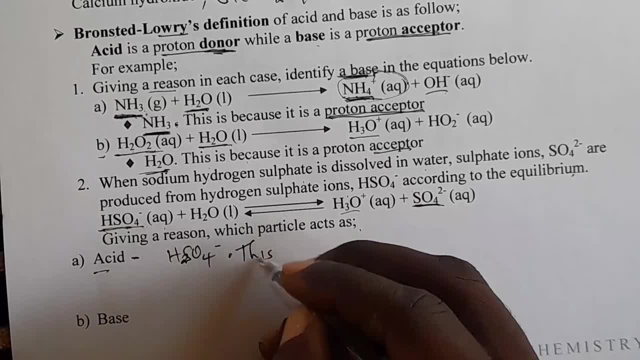 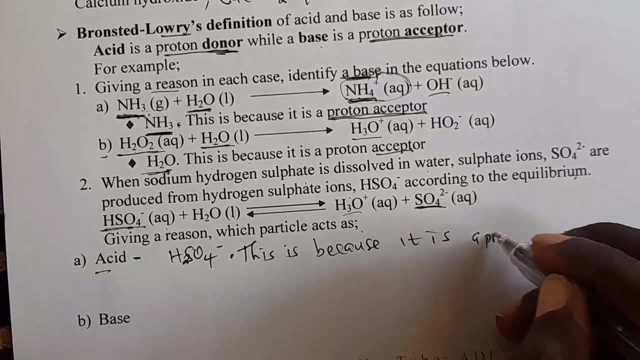 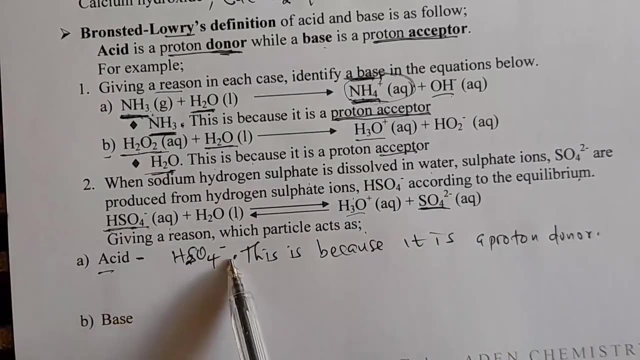 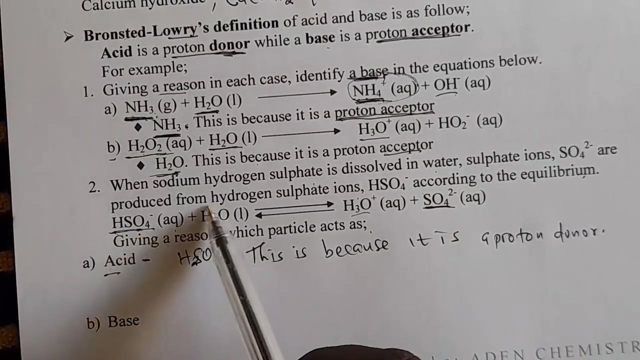 ion. first of what is the reason? this is because this is because it is a proton donor. a proton donor, let's go. we can also say reason: this is because hydrogen sulfate ion donates the proton to water to form sulfate ions. you can see that, if you don't want to say it's a proton. 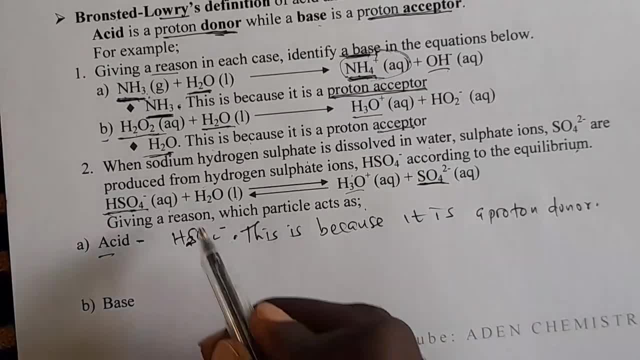 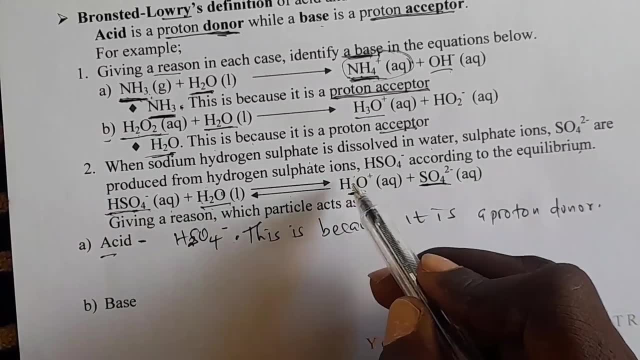 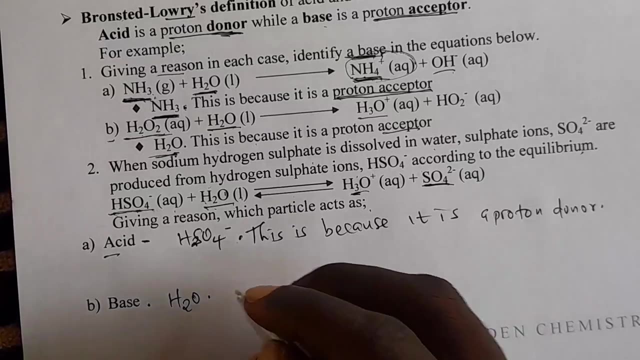 donor. let's go to abyss. so abyss it is water because it is h2o. then you see here it has accepted the hydrogen atom or hydrogen proton to form hydronium ion. so we are going to see: here is water, is our answer. reason, because it is a proton acceptor. it is. 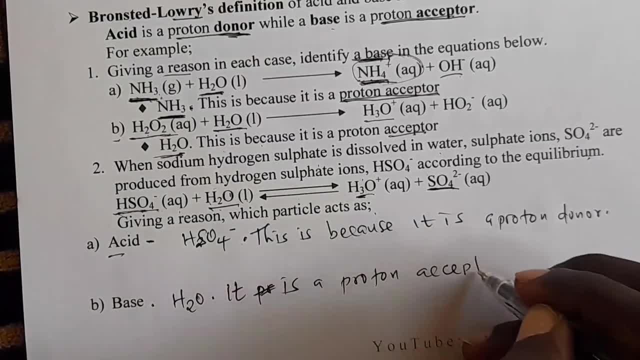 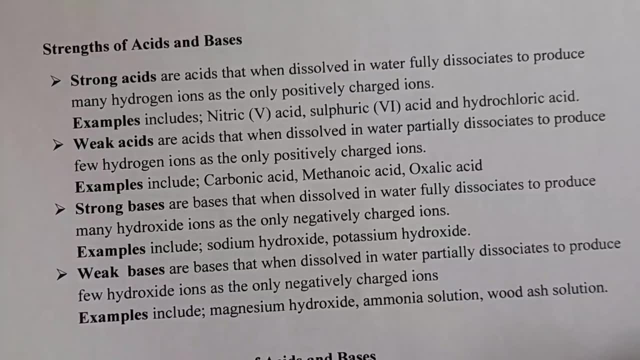 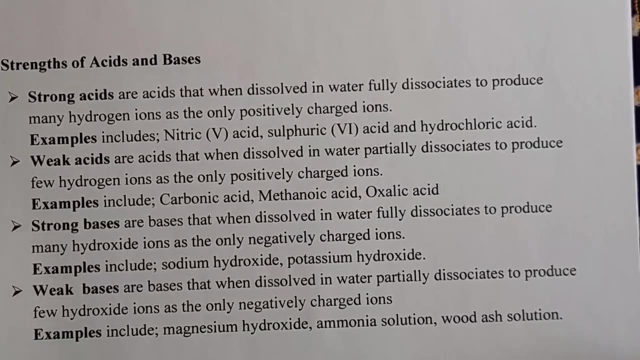 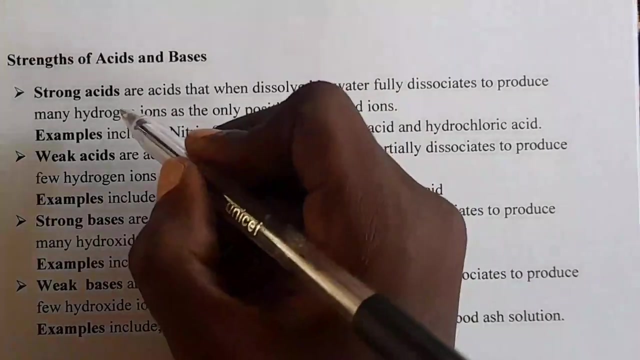 a proton acceptor. okay, after that let's just try to go to see the strength of acids and bases. so we want to define some terms like what is a strong acid, what is a weak acid, what's a strong base, what is a weak base? so let's start with strong acid. if you know one definition, then that: 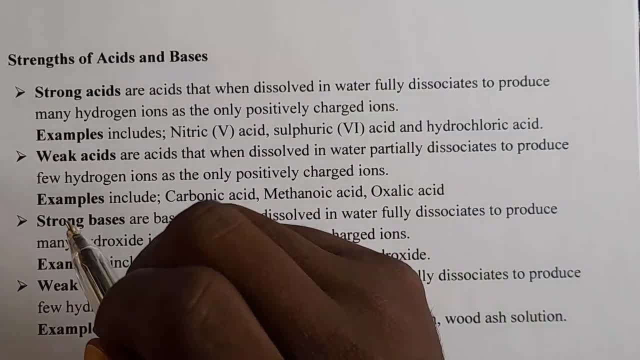 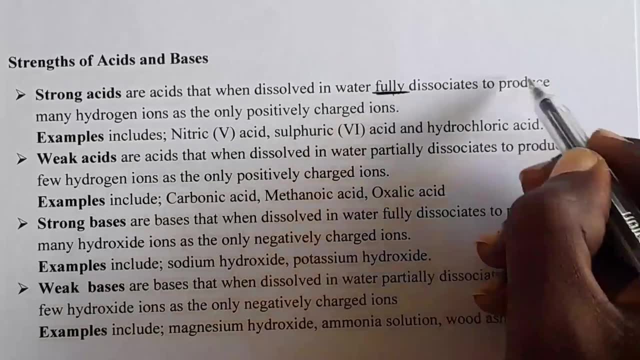 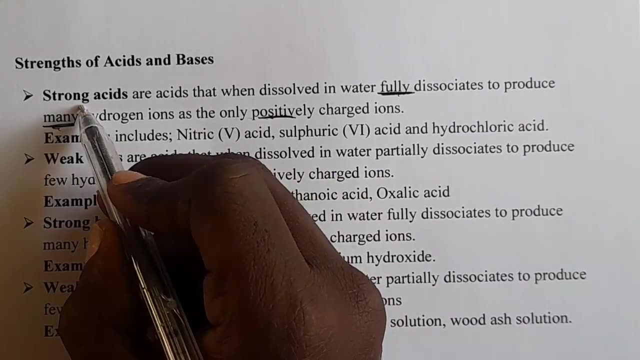 means you can know the others just by changing some small thing. you can know the others just by changing some small thing. so what is strong acids are acids that, when dissolved in water, fully dissociate. so this one here to produce many, this other one again, many hydrogen ions as the only positively judged ions. so we are talking about acid. that means we 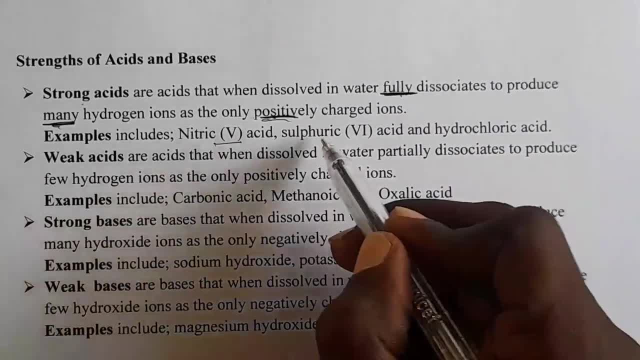 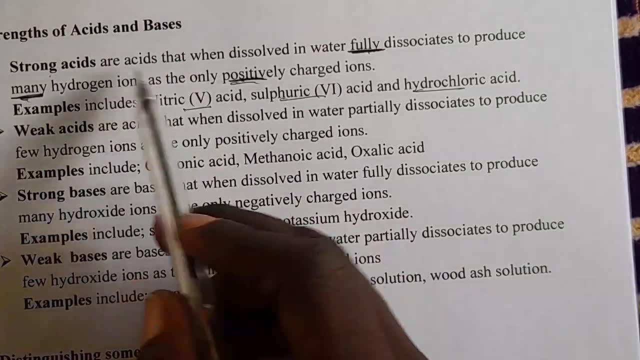 are supposed to have only positively judged ions. example: nitric sulfate, sulfated acid. we are having hydrochloric acid. okay, let's go to weak acids. what are weak acids? you just check from strong acids. where you see fully, you change to partially. where you see many, you change to. 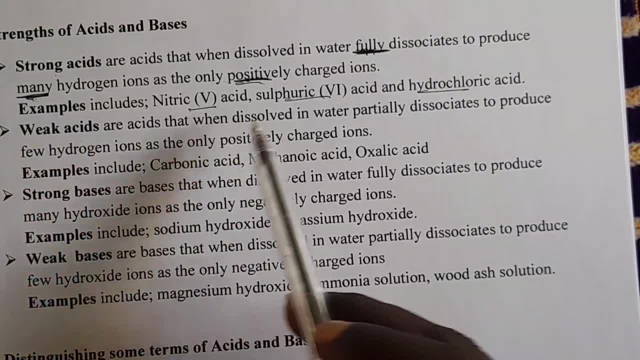 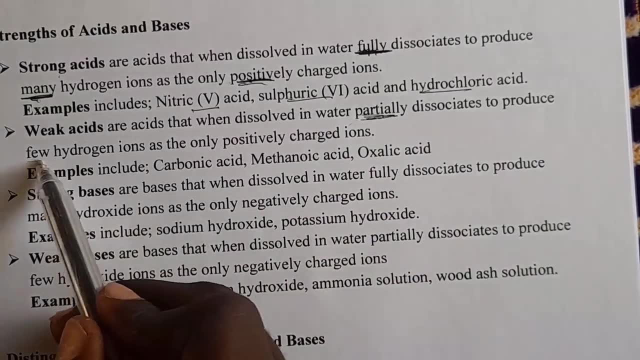 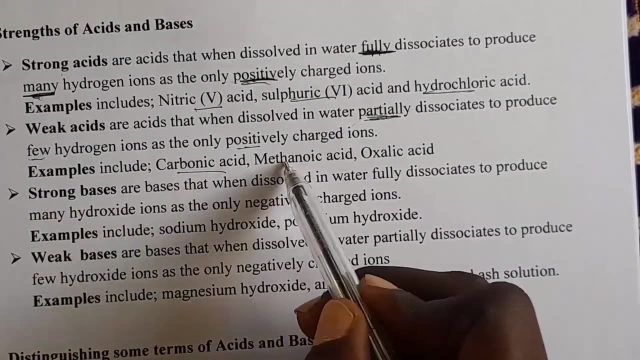 few hydrogen ions. so weak acids are acids that, when dissolved in water, partially dissociates, so, instead of fully partially dissociates, to produce or to form few hydrogen ions instead of many hydrogen ions. as the only positive hydrogen ions examples: carbonic acid, methanolic acid, oxalic. 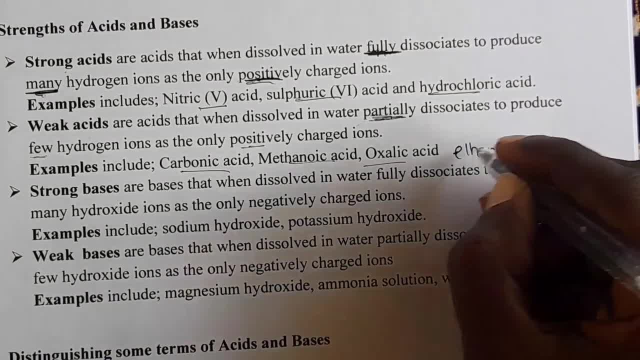 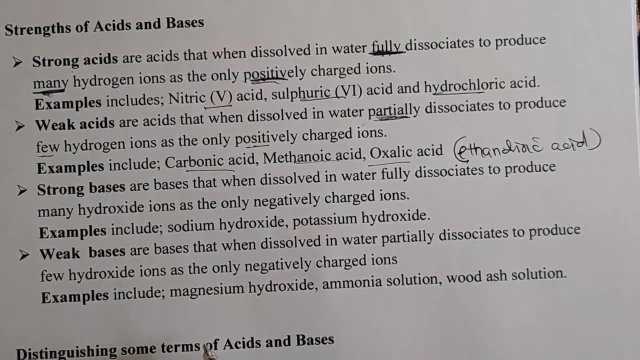 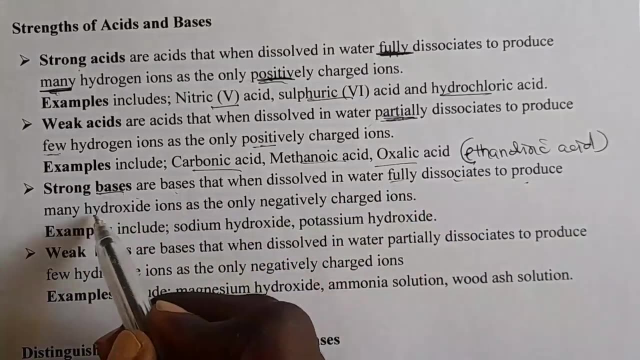 acid or ethandioic acid, ethan, ethan dioic acid. oxalic acid and ethan dioic acid are just one and the same, so let's got strong bases. so what are strong bases? are bases that, when dissolved in water, fully dissociate to produce many hydroxyl ion as the only negatively judged. so what are you? 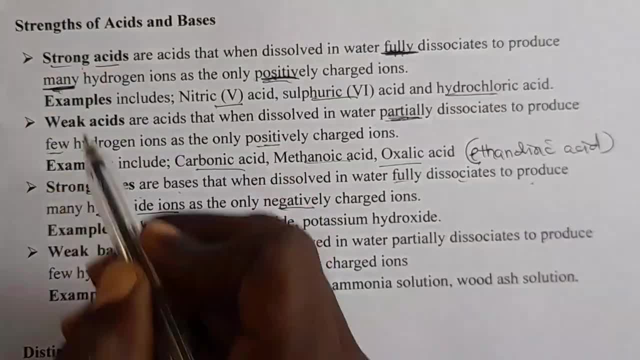 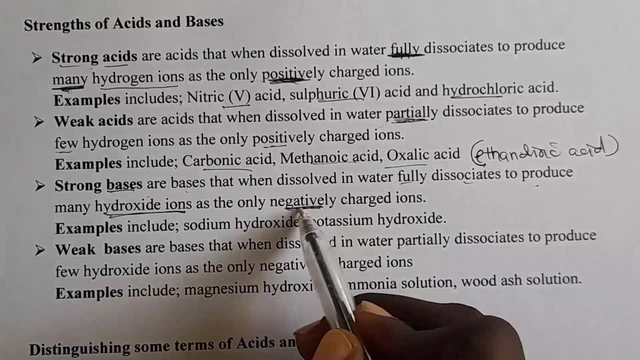 going to change. if you know what strong acid is, two side only: where you have hydrogen ions, you make hydroxyl ions. where you have positively judged ions, you make negatively judged ions. so your definition will be correct. you know only strong acid. you can know the others examples. 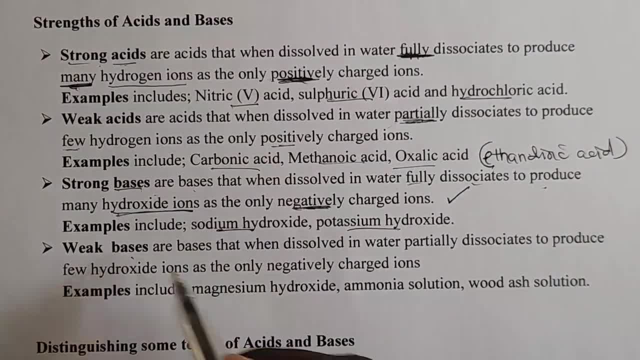 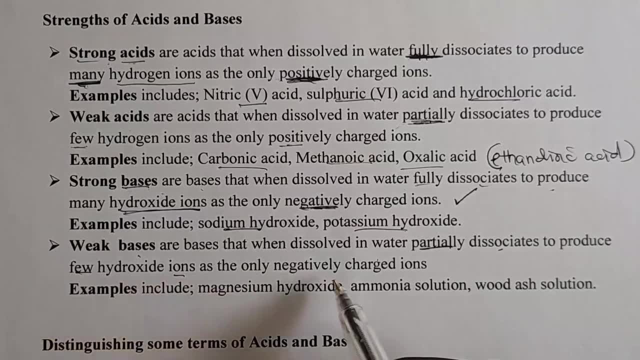 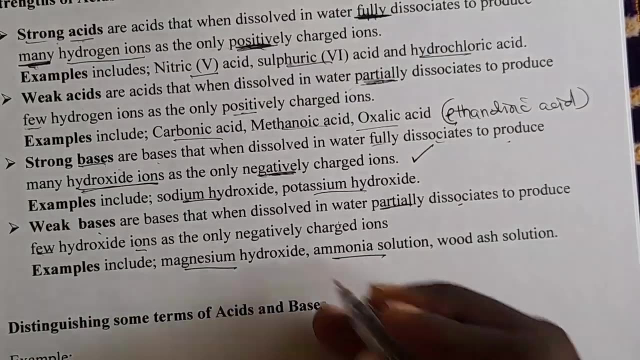 include sodium hydroxide, but also hydroxide. weak acids are acids that, when dissolved in water, partially dissociates to produce few or fewer hydrogen ions as the only negatively judged ions. examples include magnesium hydroxide, ammonia solution or ammonium hydroxide. you can see that ammonia solution and ammonium hydroxide are just 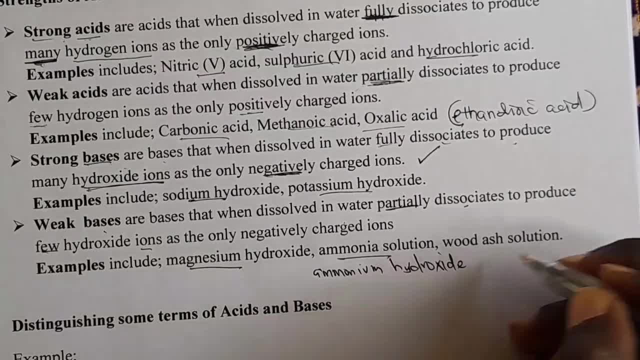 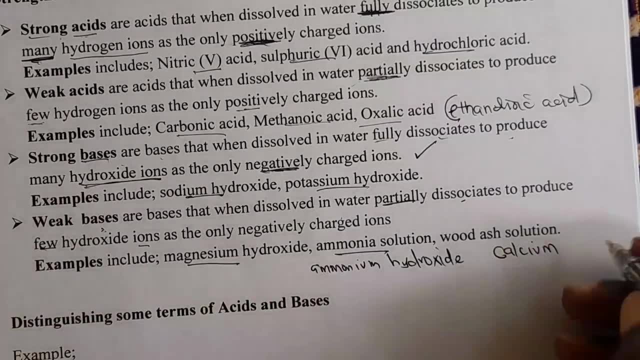 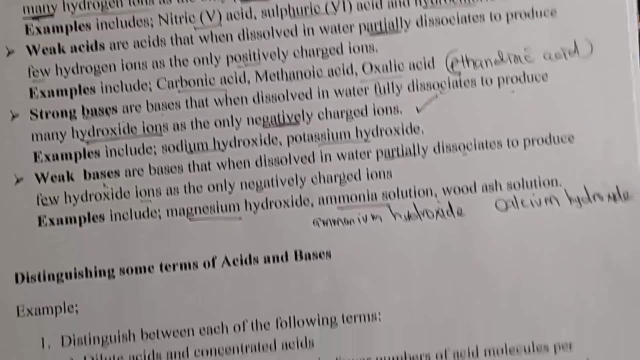 one and the same. we have food wood ash solution and you can put another example like calcium hydroxide, which is a weak base: calcium hydroxide, calcium hydroxide. so thereafter let's just try to go distinguishing some terms of acids and bases. example: you can be told distinguish between: 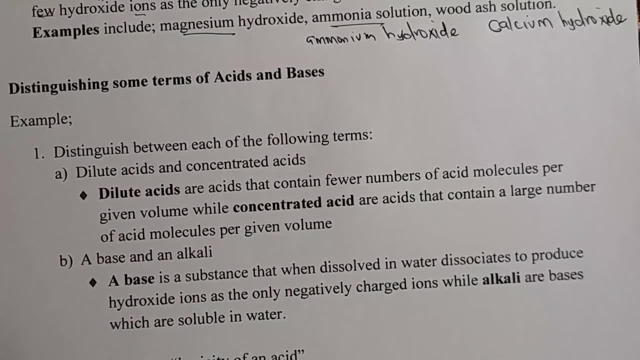 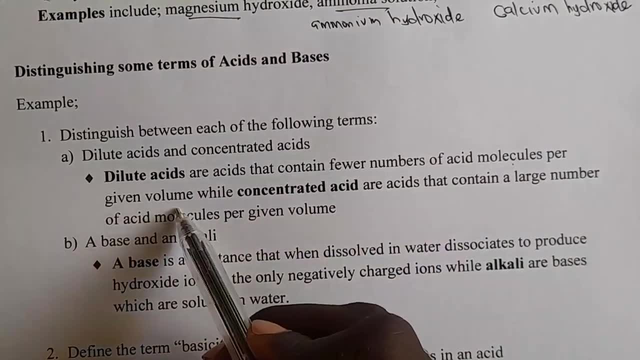 the following terms. so we are having one dilute acid and concentrated acid. what are dilute acids? so dilute acids are acids that contain few number of acid molecules by giving volume. what about concentrated acid? are acids that contain large number of acid molecules by giving volume.